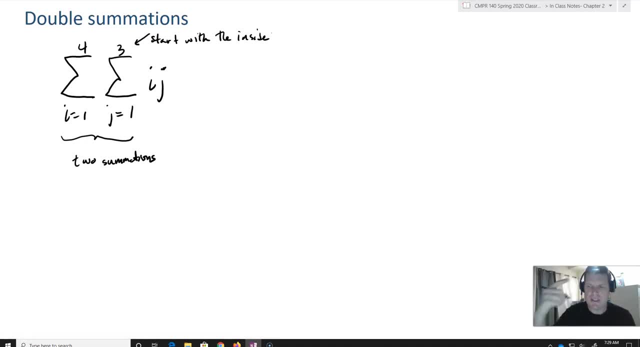 you know, taking the value for j. each and every time, what we've got to do is we've actually got to write out. in this case, we've got a couple of summations that we're going to write out. So we're going to substitute one in for j and then two in for j and three into j, but then that. 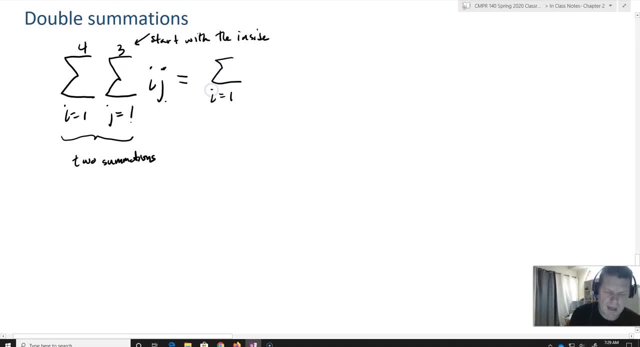 means that we're going to end up with the sum i equals one up to four of, in this case one i. So that's when we're going to have the sum of i equals one up to four of, in this case one i. j equals one plus the sum i equals one up to four of two i. that's for j equals two. 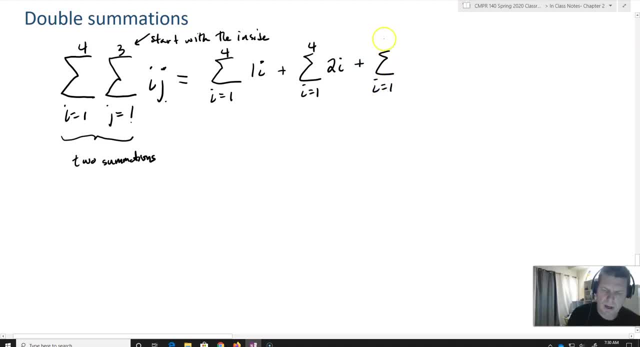 plus the sum, i equals one up to four for three i. So what you're going to notice is that we're actually going to take, we're going to iterate this summation, we're going to iterate the outer summation as many times as we actually have the inner summation. 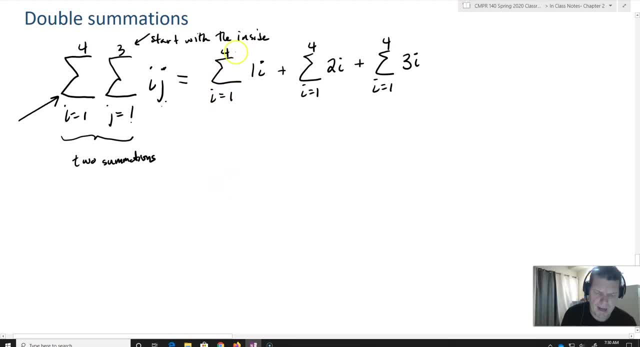 All right, and so now we're going to have to evaluate Each one of them. i equals one up to four of i all right is going to be one plus two plus three plus four plus, and then now we're going to take two times i plus. so that's the first summation. 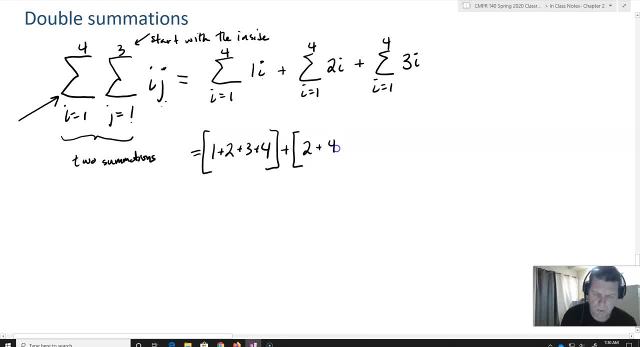 plus two plus four plus six plus eight. that's the second summation. and then we have the third summation, which is going to be three plus six plus nine plus twelve. Okay, so you'll notice that what we've done now is we've taken that outer summation right with the 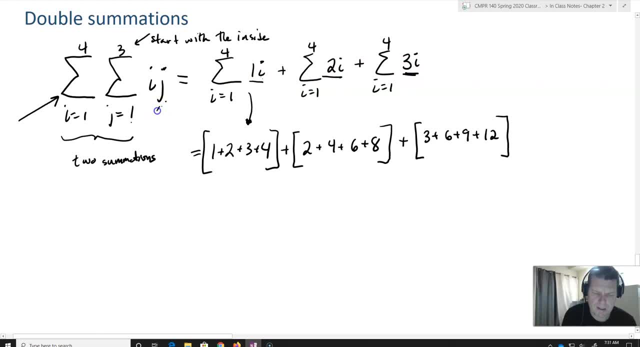 new sequence, the new sequence that incorporates all of our values for j. so this one is three plus three, that's ten plus, and this is going to be twenty, and this will be plus thirty, okay, which equals sixty. and there you go Some cool stuff we can do with summations. actually, that might make this a little bit easier is to notice that say, for example, notice how ten, okay, twenty and thirty they're related, right? 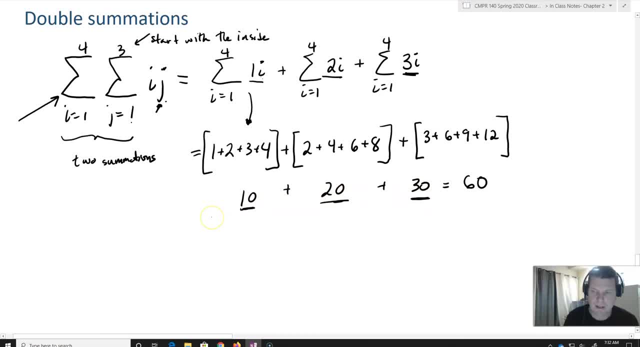 Twenty is two times ten and thirty is three times ten, right? so if you kind of remember from your pre-calculus class, you might remember that if i have the sum- excuse me, the sum i equals one up to four of two i I can actually pull that between these two problans here. 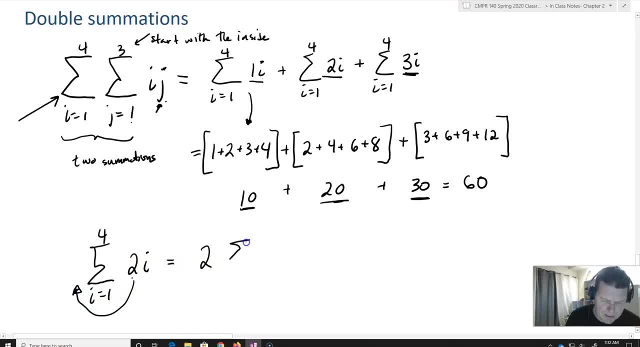 pull that scalar out of the summation and then I can make it 2 times the sum. i equals 1 up to 4 of i. Now I know what the summation of i is. The summation of i ends up being 10, so that means that 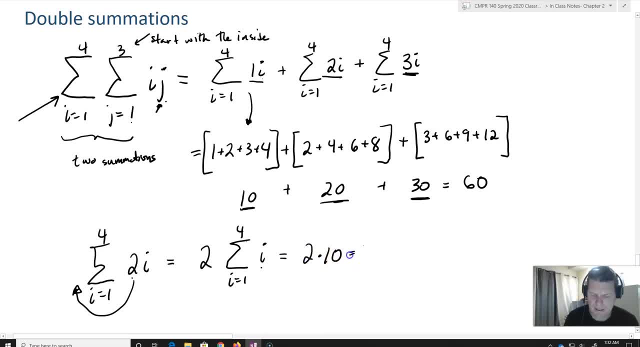 this is just going to be 2 times 10 and that's 20.. It's kind of a little cool little thing that you can do when you're working with your summations. Now let's take a look at another example. Let's. 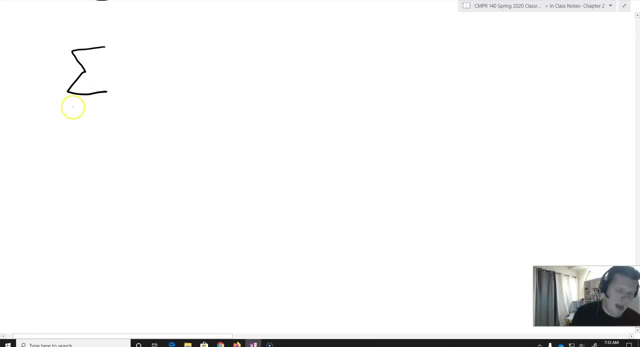 look at another example of a double summation. So we're going to take the summation i equals 1 up to 3 times the summation of i equals 1 or j equals 1 up to 2 of i minus j. So again, we're going to do the inner summation first. All right, nice that there's not too many. 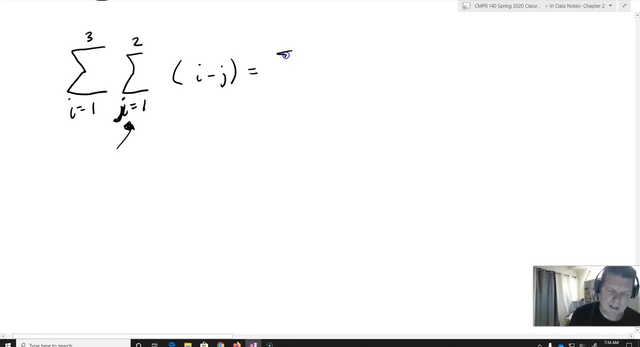 of them, and so this is going to end up equaling, right: the sum i equals 1 up to 3 of i minus 1, plus the sum i equals 1 up to 3 of i minus 2.. Okay, then we're just going to go out. 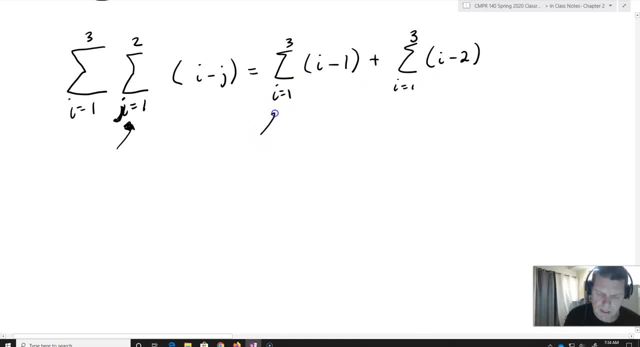 and evaluate each sum right. So for this first sum, this guy right here, that's going to give me 1 minus 1 plus 2 minus 1 plus 3 minus 1, and then the second sum is going to be plus 1 minus 2 plus 2 minus 2 plus 3 minus 2.. Okay, so we start with our inside. All right, we evaluate. 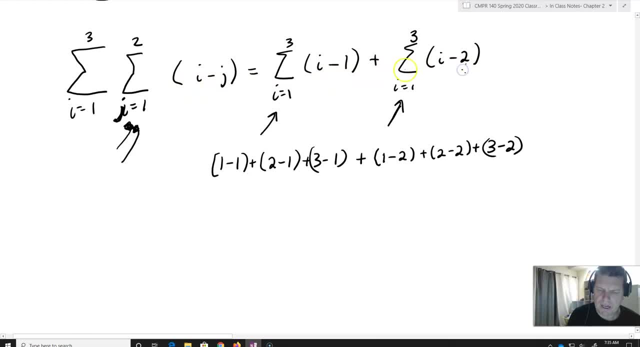 that, plugging in basically our values for j for each one of the summations and then we'll evaluate the sum in each term. So this will be 0 plus 1 plus 2 plus negative, 1 plus 0 plus 1.. That's going.